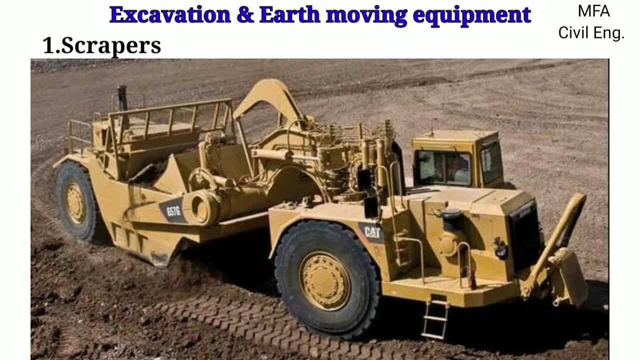 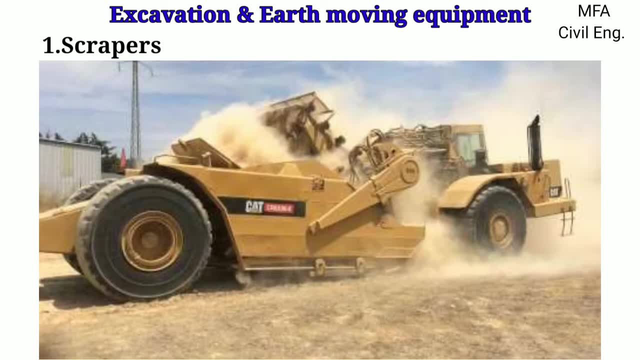 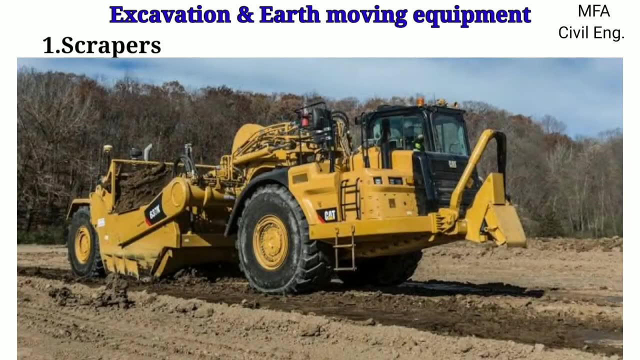 through scraping the ground and carries the load over the required distance, discharging and spreading the materials, and then returns back to the pit for the next load. Therefore it does not depend on other equipment. The wheels of the machines cause some compaction of the soil. The ability of these machines 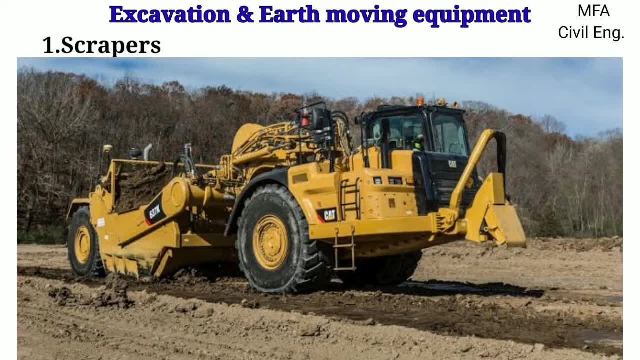 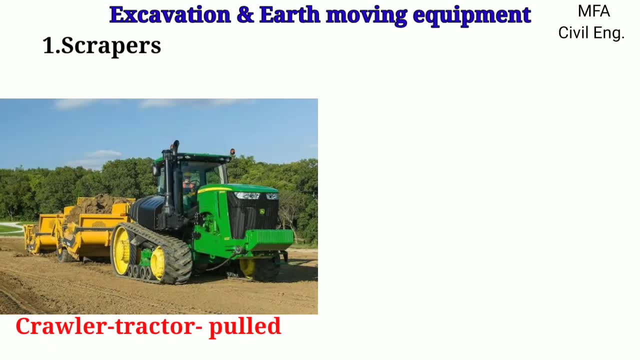 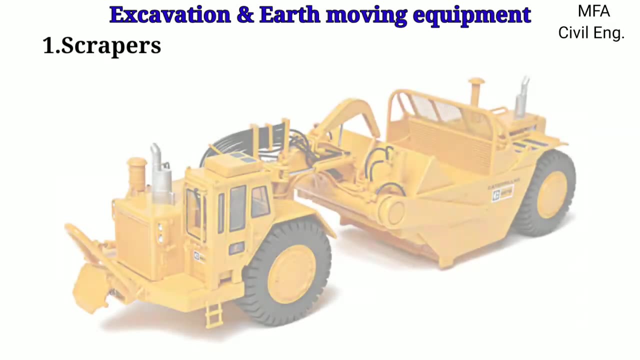 to deposit the load is a uniform thick layer facilitate the succeeding spreading operation. Scrapers are classified as crawler tractor-pulled and wheel tractor-pulled, Depend on the type of the tractor used to pull them. The capacity of the scrapper may be specified as the heap. 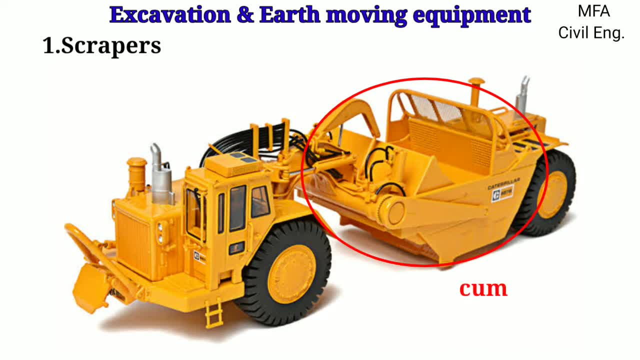 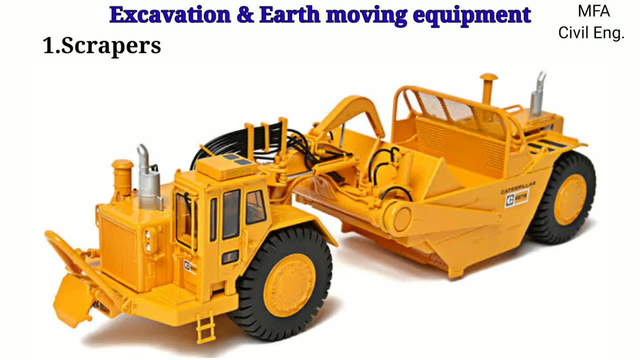 capacity. The scrapper may be classified as the heap capacity of the bowl 10.. The scrapper's impact on the held Hill Crouch Ex-Praise. in cubic Shafts and All meter. Scrappers are either cable or the hydraulic operated. The basic part of the scrappers are 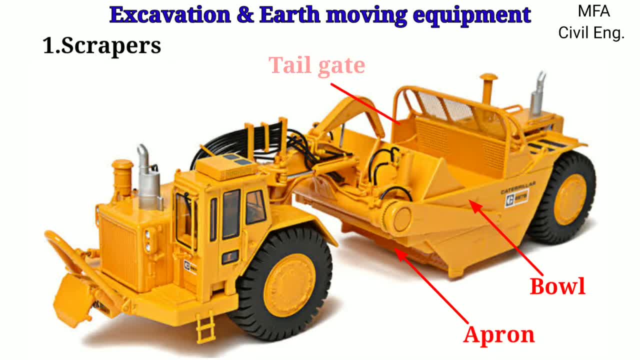 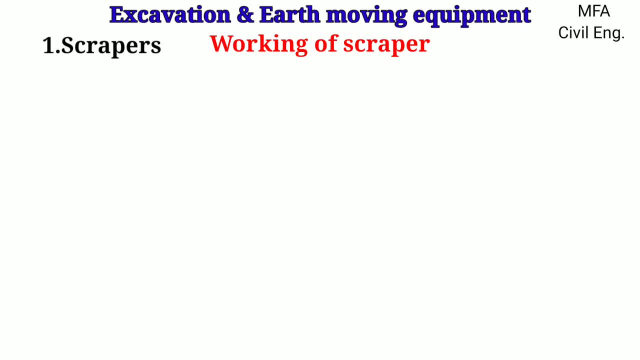 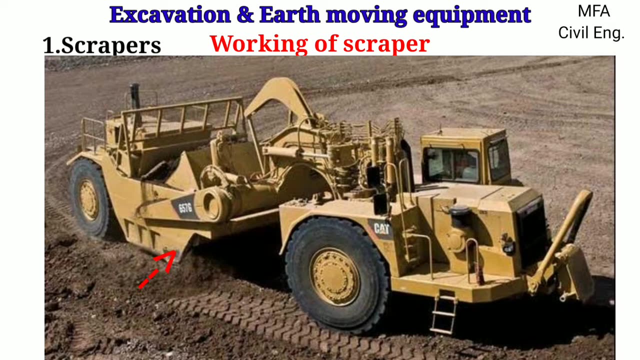 the bowl apron and the tailgate or ejectors. The working operation of the scrappers is in such a way: the loading operation of the scrapper is done by lowering the front end of the bowl till the cutting edge enter the ground. Simultaneously, the front apron is raised to provide an opening. 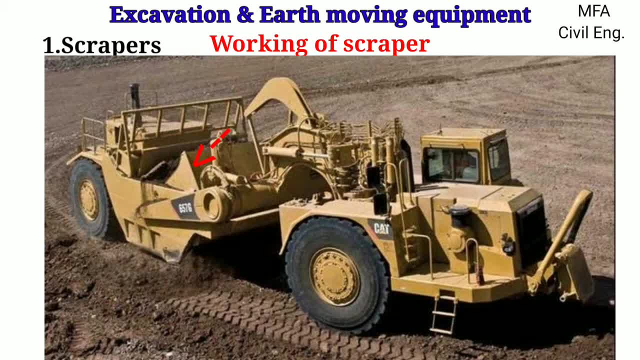 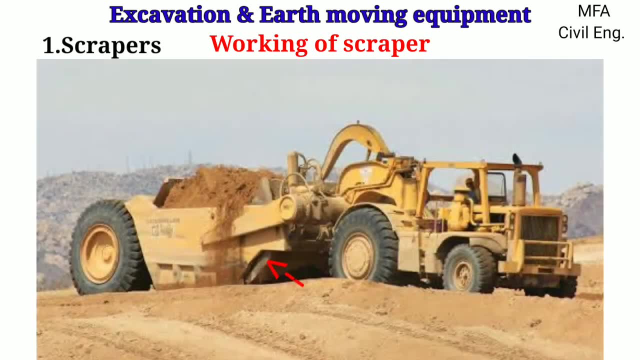 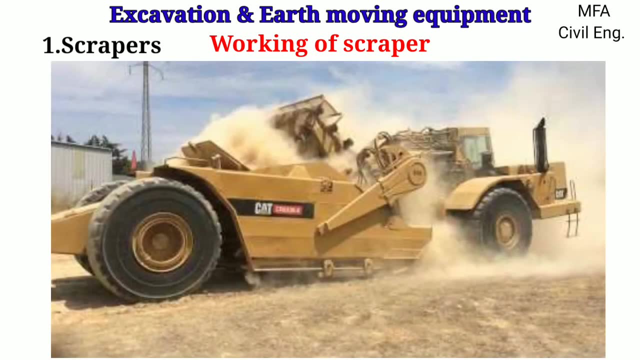 slot through which the earth flow into the bowl. As the scrapper move forward, the earth is forced into the bowl, The cutting edge is raised and the apron is lowered to prevent spillage during the hauling. The dumping operation is done by lowering the cutting edge to the 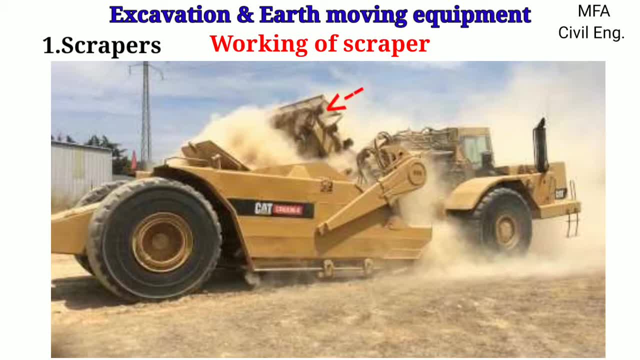 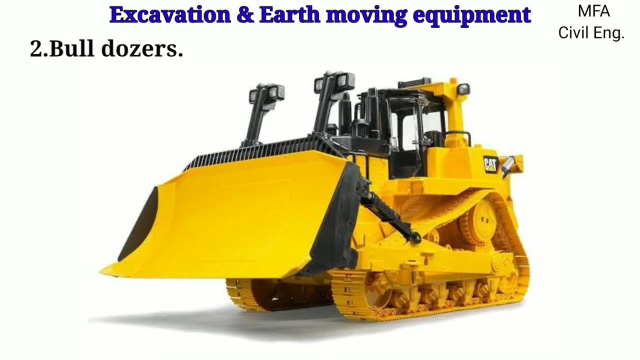 desired height above the frame. The scrapper is then allowed to move back to the bowl, raising the apron and forcing the earth out between the plates and the apron by means of the movable ejectors mounted at the rear of the bowl. Bulldozers are commonly used in a construction project. It is essentially a heavy steel blade. 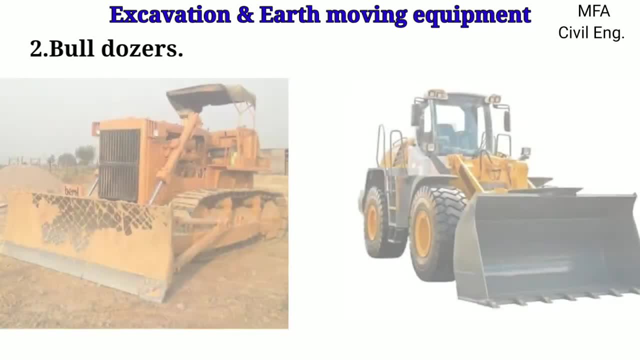 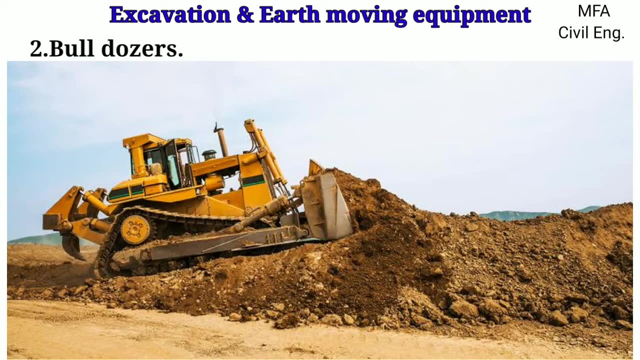 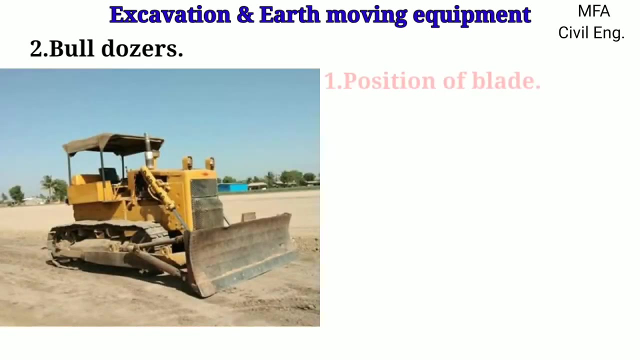 which is mounted on the front of the tractor. The tractor can be a crawler or the wheel type. The heavy blade attached to the tractor pushes the material from one place to another to another. Bulldozers are basically classified on the basis of the position of the blades based. 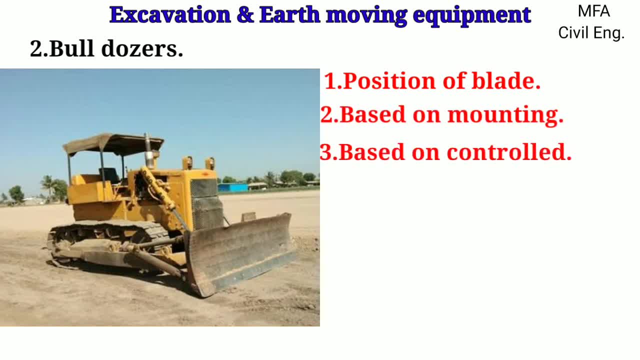 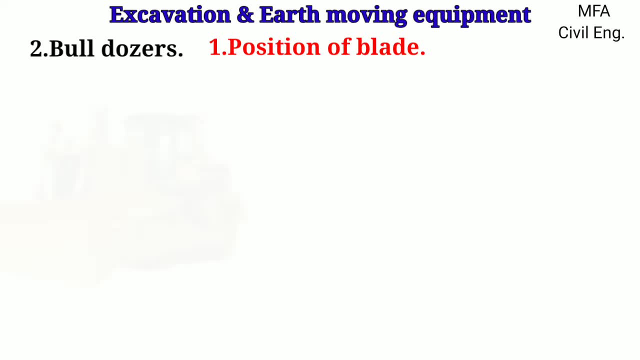 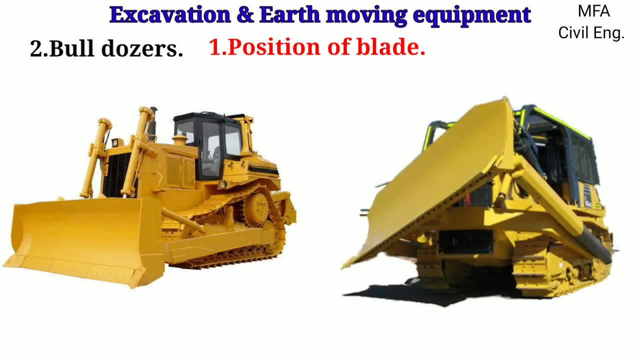 on the mounting and based on the control. Based on the position of the blades. bulldozers are further classified into two types, like bulldozers with the blade perpendicular to the direction of movement, and bulldozers in which the blade is set at an angle to the direction of movement. 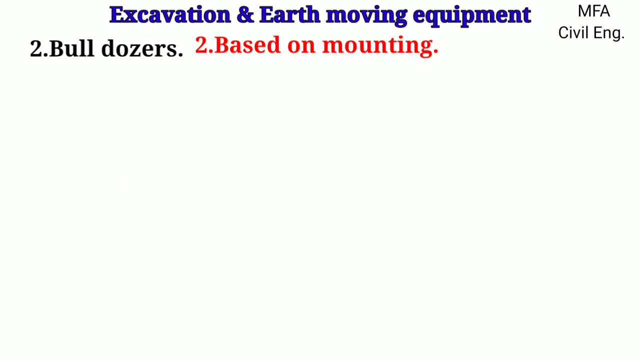 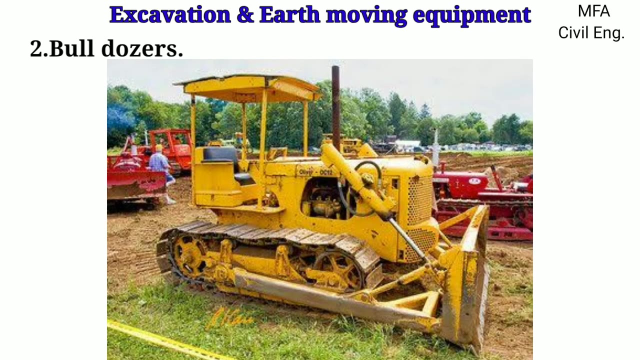 Based on mounting, bulldozers are further classified as wheel-mounted and crawler-mounted. Based on the control, the bulldozers are further classified as cable-controlled and hydraulic-controlled. The earth-moving bulldozers consist of a heavy blade of somewhat concave profile. 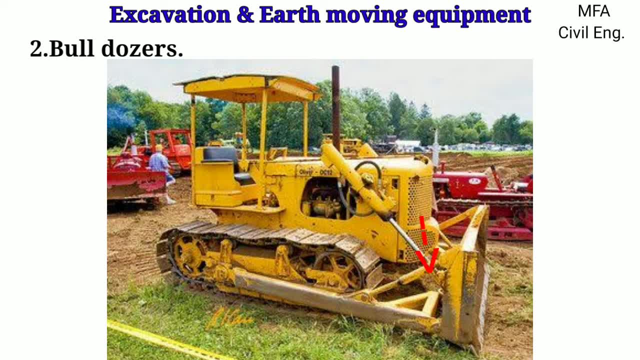 The blade is attached to the body of the truck. The blade is held at a lower edge on the two heavily built push arms which are hinged to the track frame of the tractors. The top of the blade is supported by the two brace arms attached to the push arm. 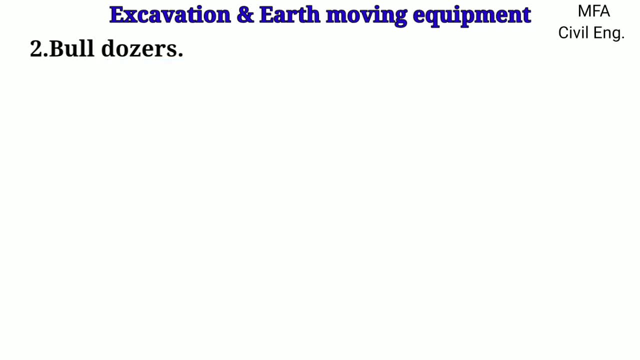 The blade is projecting ahead at the bottom. Bulldozers are mainly used for various operations like for spreading the earth field, for opening up a pilot road through a mountainous and rocky terrain, cleaning construction sites, maintaining haul roads, cleaning land from trees and stumps, bag-filling trenches at 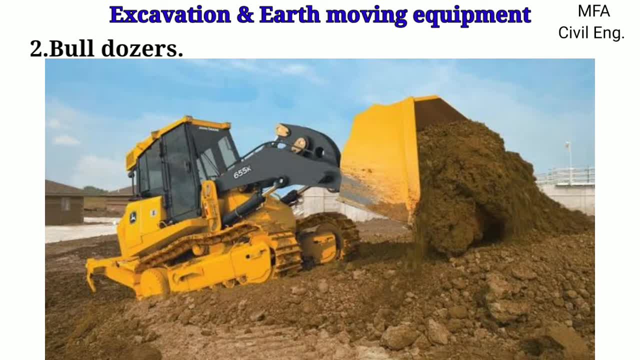 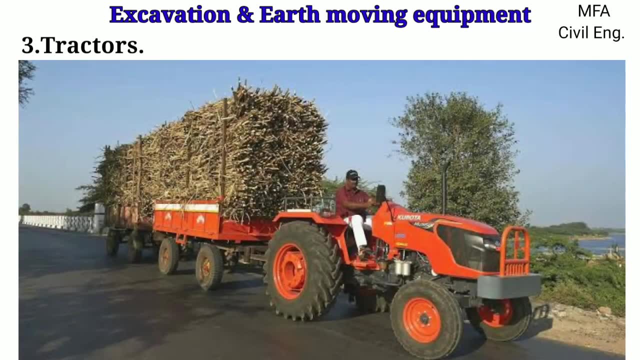 the construction site by dragging the earth from one place to another. Tractors are the multipurpose machines used mainly for pulling and pushing the other equipment or the heavy load. They are also used for agricultural purposes. Bulldozers are mainly used for pulling and pushing other equipment or heavy loads. 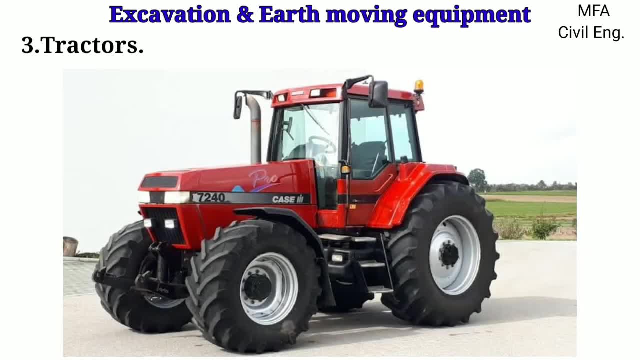 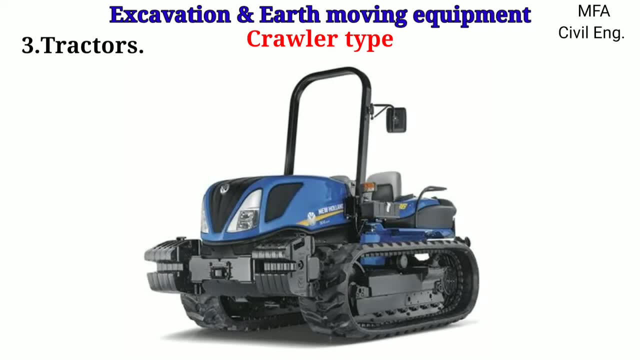 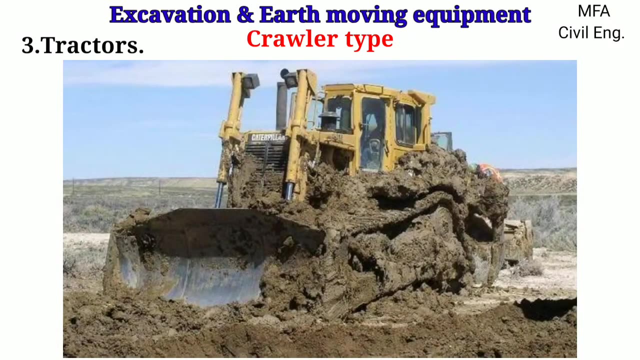 They are also used for agricultural purposes. Tractors may be classified as crawler type and the wheel type. Crawler type tractors is a versatile equipment used to move bulldozers, scrapers and wagons on the rough road. The crawler has a chain by which this tractor can be very effective, even in case of the